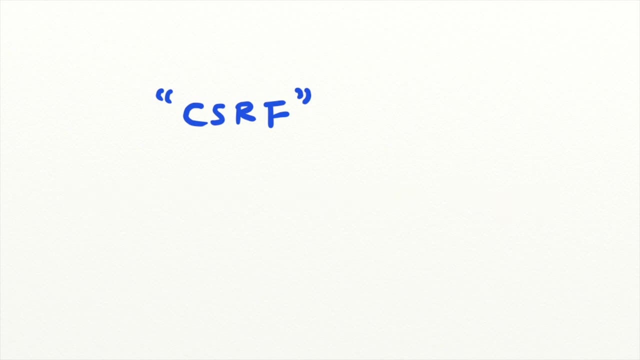 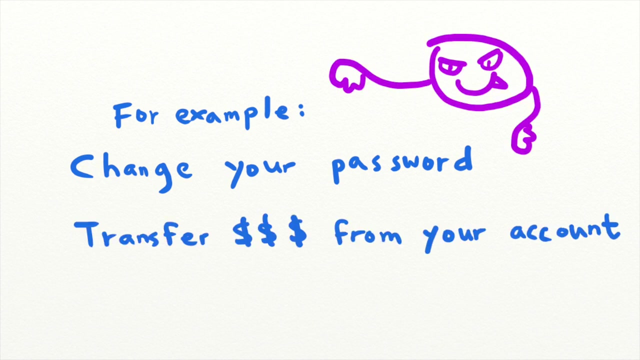 CSRF, or cross-site request forgery, is a technique that allows hackers to carry out unwanted actions on the victim's behalf. For example, an attacker might be able to change your password or transfer money from your bank account without your permission, But how is this attack possible? Before we dive into the mechanisms of a CSRF, 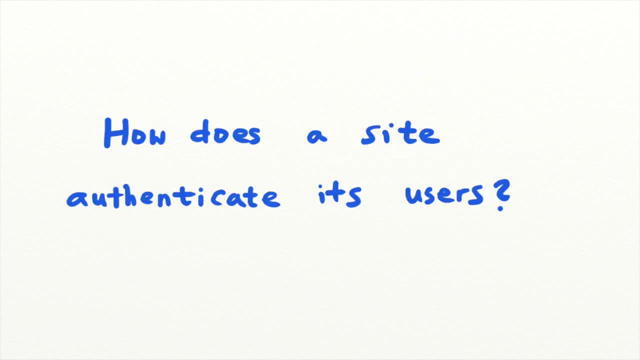 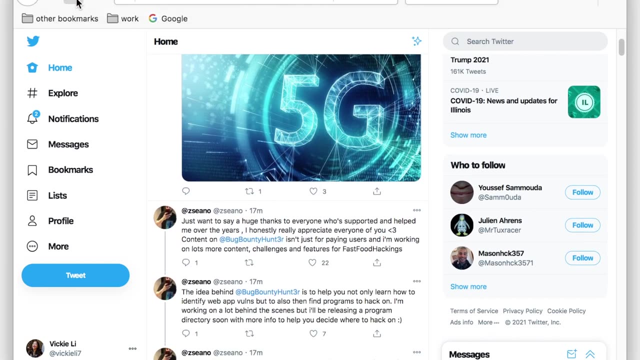 attack. let's first talk about what is a cross-site request forgery. In a cross-site attack, we need to understand how websites authenticate their users. Have you ever wondered: how do websites recognize me? Why is it that I don't need to log into? 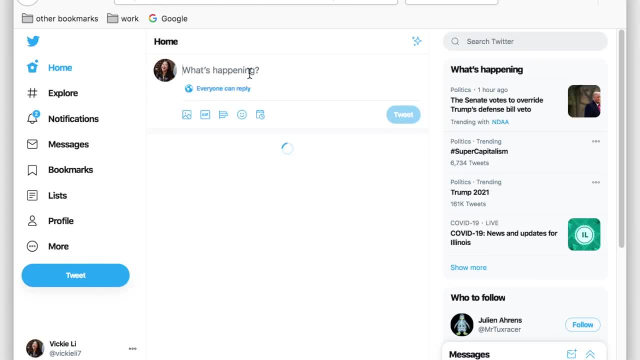 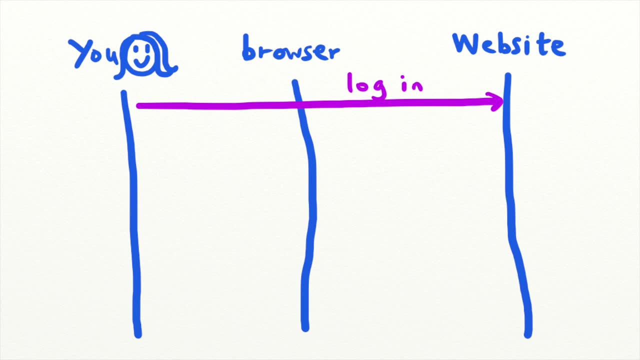 Twitter every time I check my feed When I tweet something. how does Twitter know it's me without having to ask me for my password again? Once you log onto a website, the browser that you are using stores your session cookies for that website and sends it along automatically. 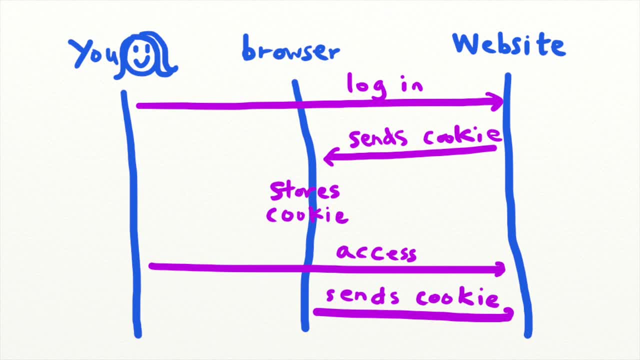 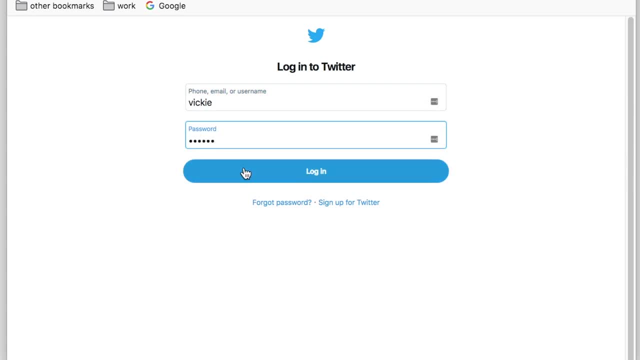 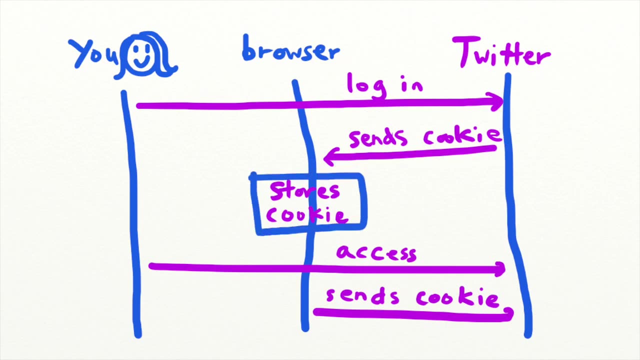 every time you communicate with that site, For example after you log into Twitter, Twitter issues a session cookie for your account. That session cookie authenticates you to Twitter. The browser that you are using receives the session cookie, stores it and sends it along with every request to Twitter. This allows you to access confidential. 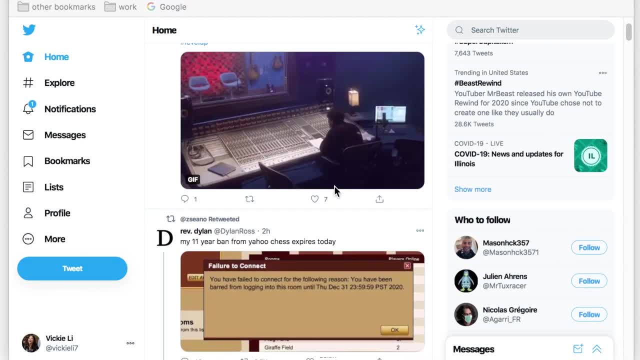 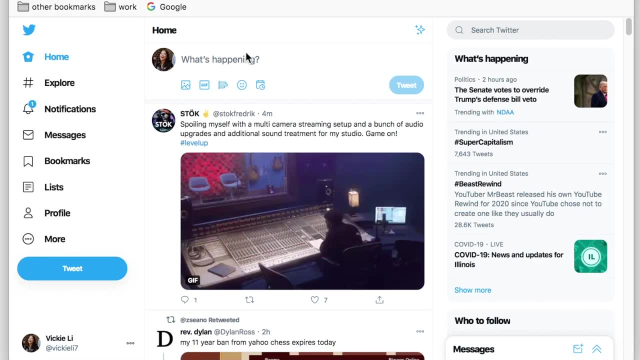 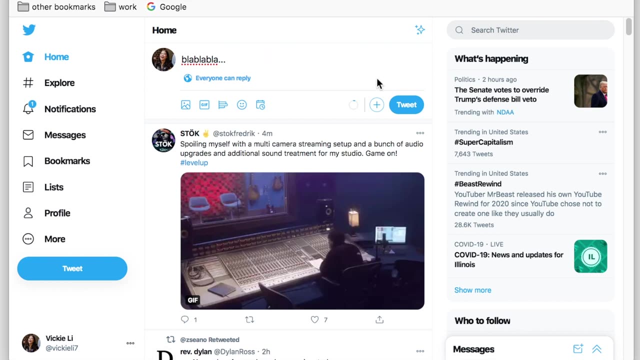 information that are only available to you and perform actions that only you should be able to do, Like reading your DMs and changing your account information. When you try to tweet on Twitter, your browser sends a request to Twitter with your session cookie to prove your identity and verify that you are, in fact, authorized to send the tweet. 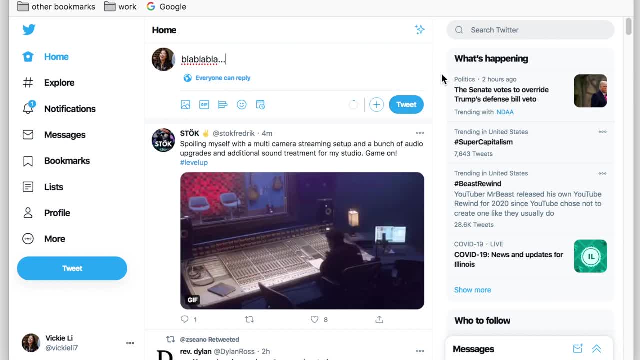 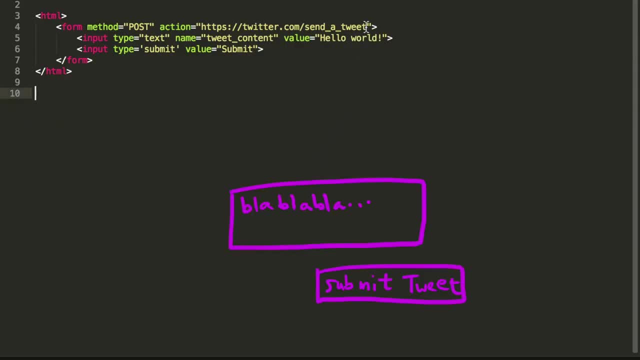 as your user account. Let's say the send a tweet HTML form looks like this: Once you click on the submit button on the page, your browser will send a request to twittercom. slash. send a tweet with your session cookie and a tweet will be sent on your behalf. 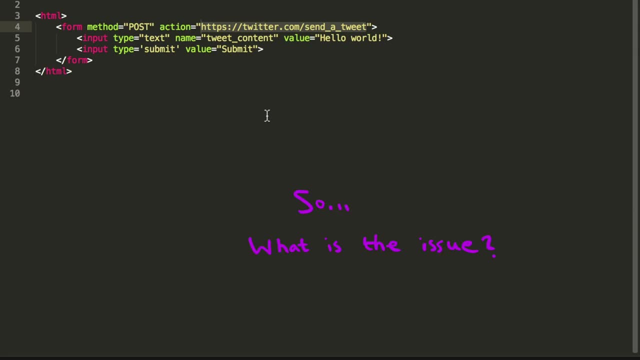 Now can you spot the issue with this functionality? A simple HTML form like this one is vulnerable because any site can submit the same request, not just twittercom. Imagine an attacker hosting her own website and on her site she hosts an auto-submitted and invisible HTML form like this one.